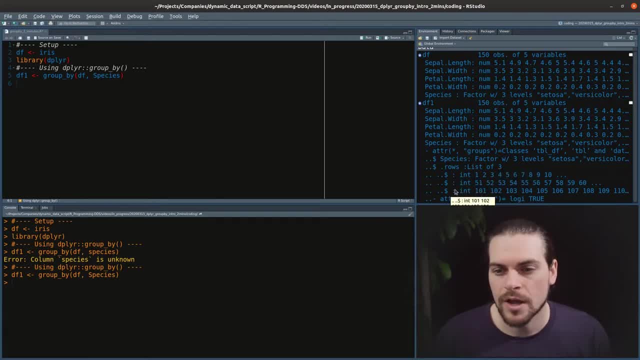 we have a list of three, and then we have some integer. Those are actually the positions of the rows that should be assigned to each of the three groups. We have three groups in this case because the species column had a factor with three levels, and so it was grouped in three groups. So why do? 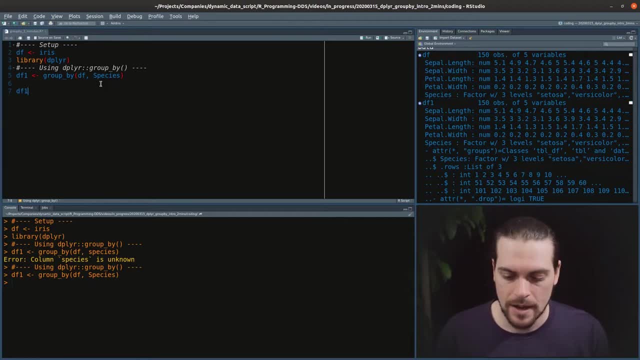 we group, And the best way to see it- see it might be with another function for which i will do a more detailed video, and so you can just click here on the link to go to this video. so the thing we can do, so i won't save the results of. 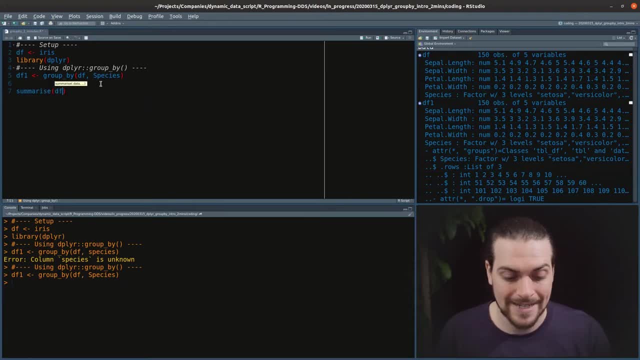 those manipulation. but let's summarize our df1. and you will see that if we summarize our df1 and then we let's, uh, let's get a mean for that summary, uh, and so if i i save the column my mean and then i do a mean of the column sepal length, you see that if i do a summary in this summary, the function 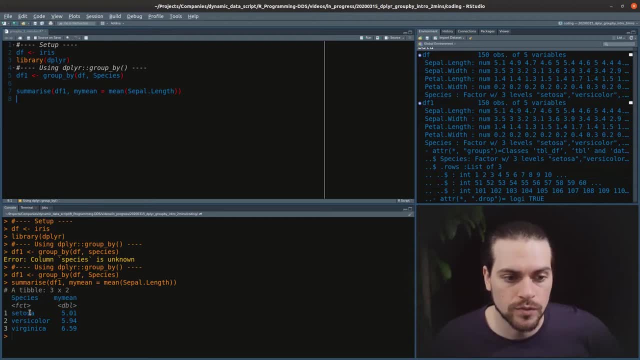 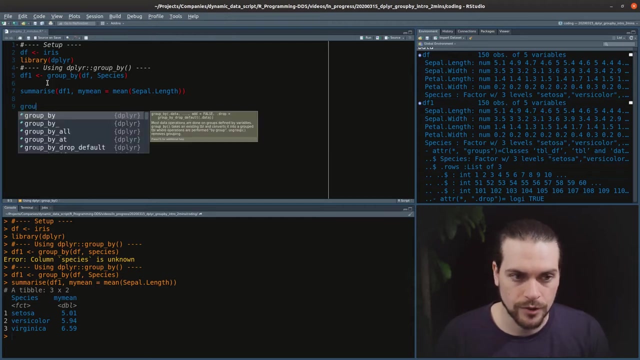 mean was applied to each groups, and so we have a result for the species cetosa, we have a result for the species versicolor and for virginica, and we have the three different means. what if i want a different group? so i can just do another group by a group by over the df1. so that's the data frame. 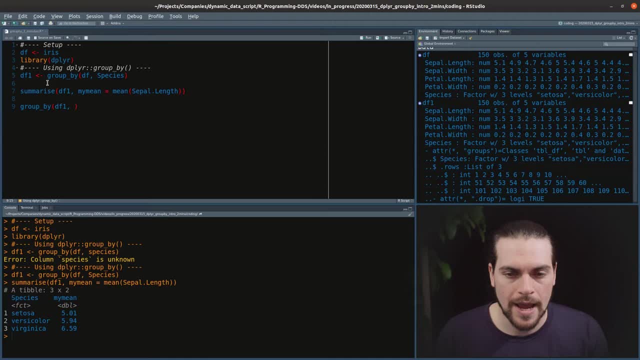 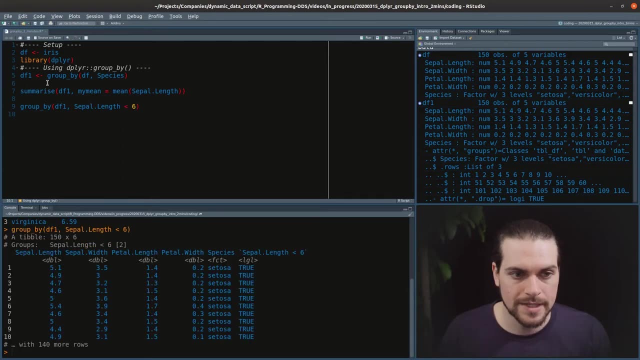 that was previously grouped in and let's say that i want to group it by sepal length smaller than six. this has grouped our data into two groups: the rows with sepal length below six and the rows with sepal length above six. if we save that into df2 and let's run the same summarize, but this time, 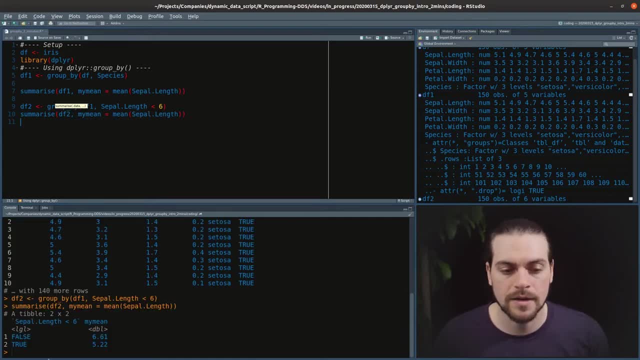 over df2 and now you see that it has summarized over two groups and, incidentally, in this case is the true or false, whether it was true that it was below six or above six- And you see that we have given the DF1 to this group by. 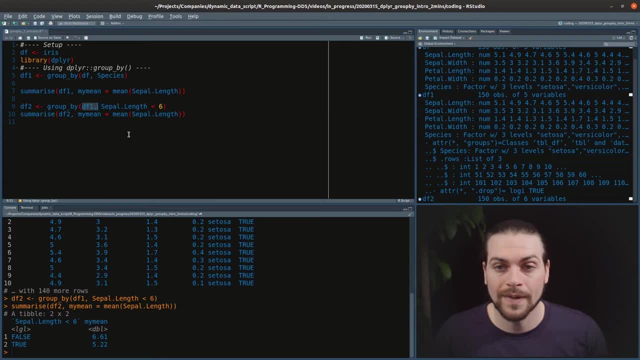 but it forgot about it, And so what that means is that whenever you do a group by on the data frame, it resets or deletes the previous grouping. If we had wanted to keep both groups, we can do both species and sepal length by only separating with a comma. 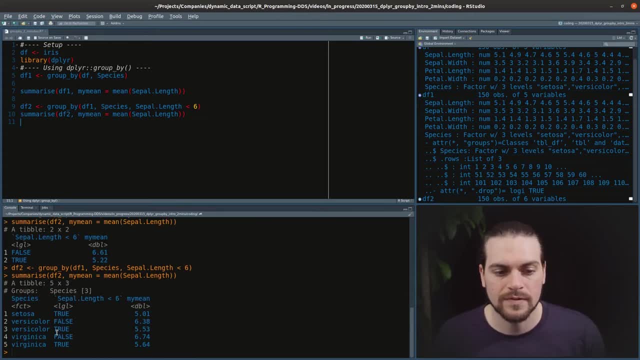 And so if I rewrite that save and you see now that we have several groups, And so for each versicolor and virginicana we have true or false, And for setosa we actually only had sepal length below six, What if I want to now have a normal summarize? 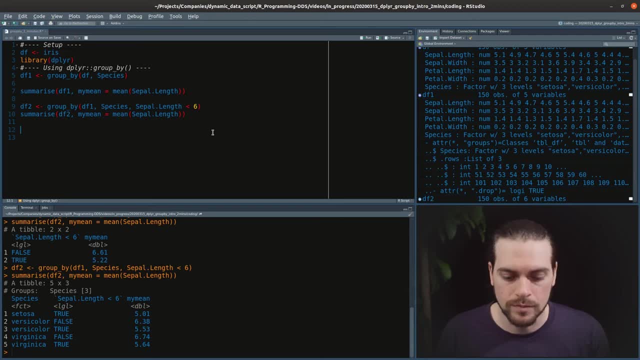 over my variable DF2, but I don't want any groups. Man, that's easy. You just have to use the function ungroup, So you can do ungroup DF2,, save that to DF3,, for example, And then let's give that. 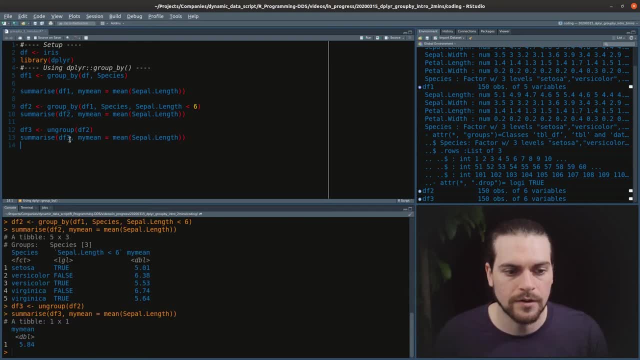 once again to our function summarize. So here you see that it has done a mean over all of the rows. I hope you enjoyed. Thanks for watching. 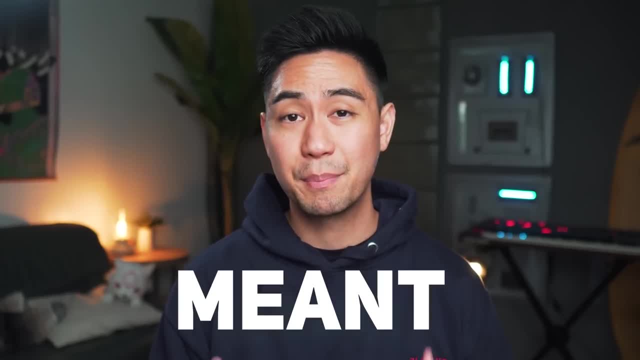 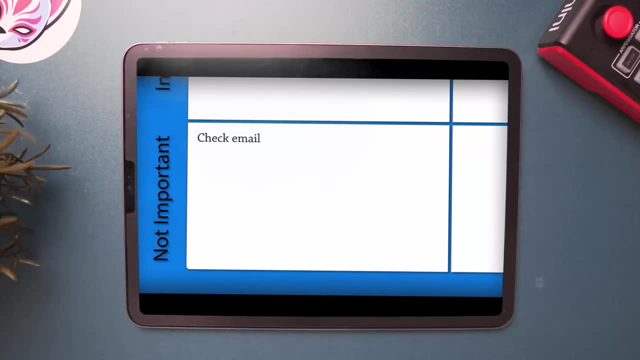 A lot of time management advice we get from productivity gurus were not meant for students, For example, delegation. Now, as somebody who runs their own business, I delegate things like checking my email or editing this video, for example. Maybe you have a lawn that you don't. 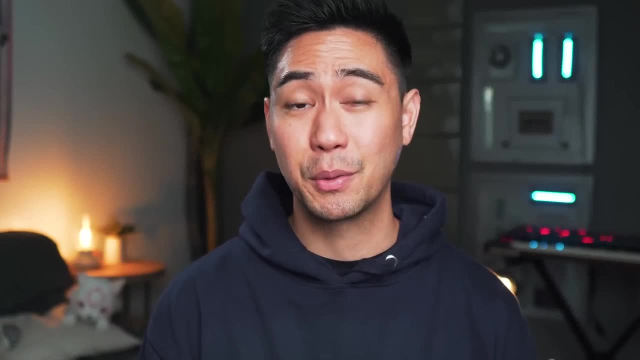 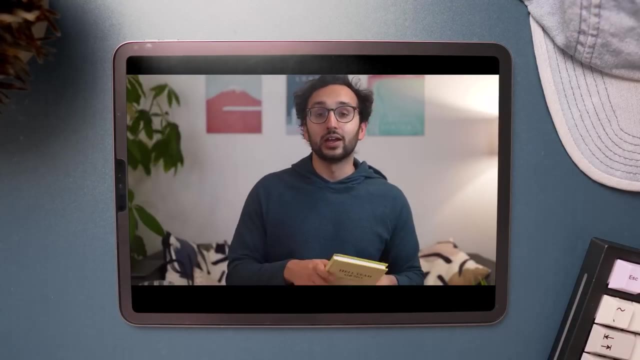 want to mow. What are students able to delegate? Are you going to have your little brother go to class for you? Another example is hell yes or no. Hell yeah or no, Just like learning to be okay with saying no to stuff If I get an email from someone saying, hey, do you want to do this thing? 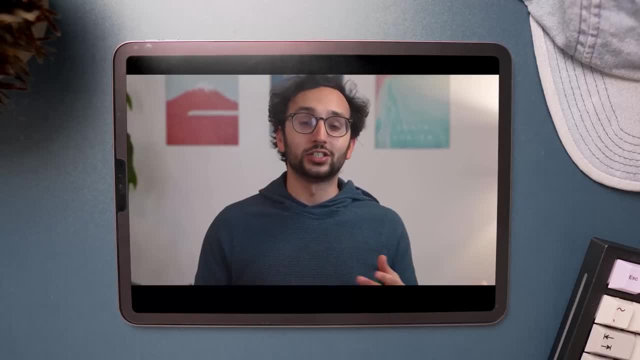 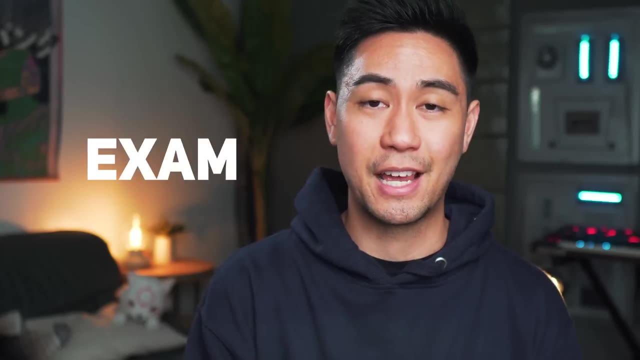 And I'm thinking: maybe it sounds kind of all right. Then my default position is going to be: no, Everything is an obligatory hell yes for a student. When can we ever say no, I don't want to take this exam, or meh, I don't feel like studying, So instead, here's a time management.